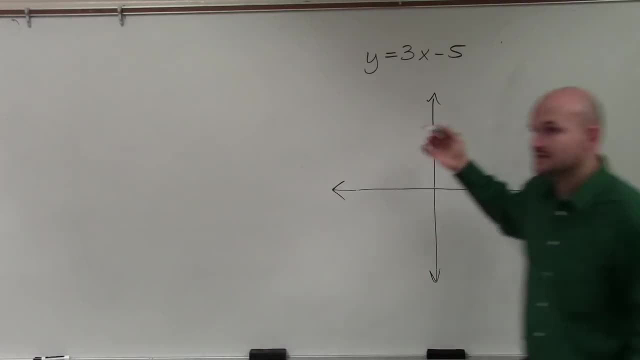 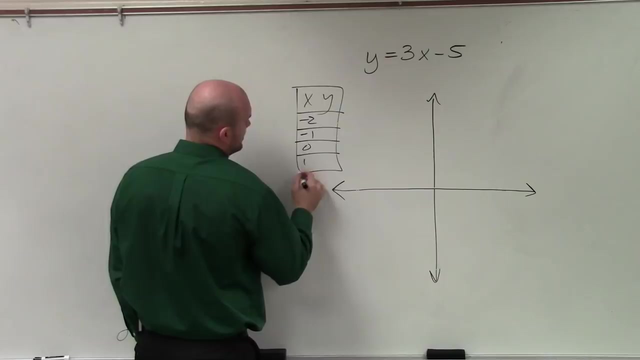 table of values. So if I wanted to graph this, I could easily set up a table of values and say, oh, here's x, y, Do negative 3, or negative 2, negative 1, 0, 1, 2.. And you'd plug in those values for x and you'd find. 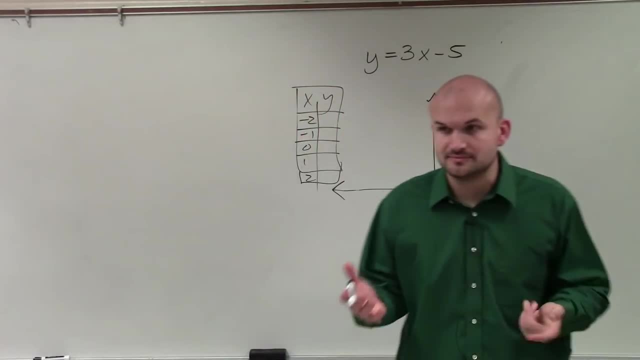 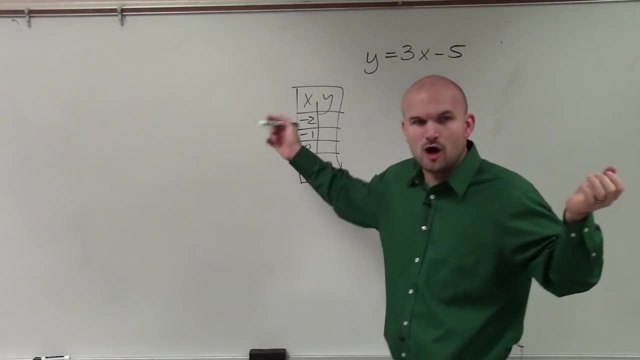 the y's right. But the nice thing about linear equations is that a linear equation is a line, right, It creates a line. So to graph this we don't need to plot all those points. If you guys noticed, with the quadratic or the cubic to kind of get the shape of the graph we needed, like all 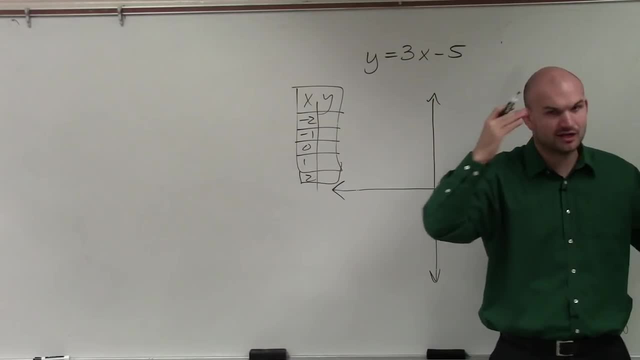 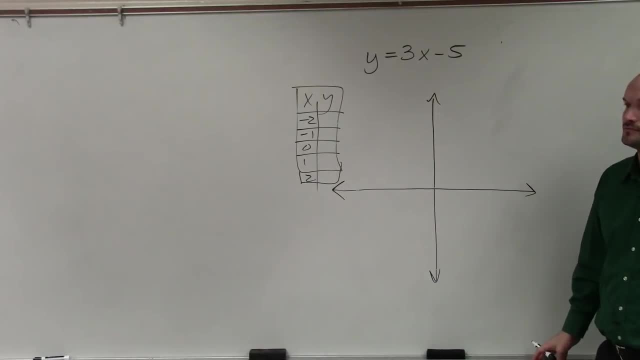 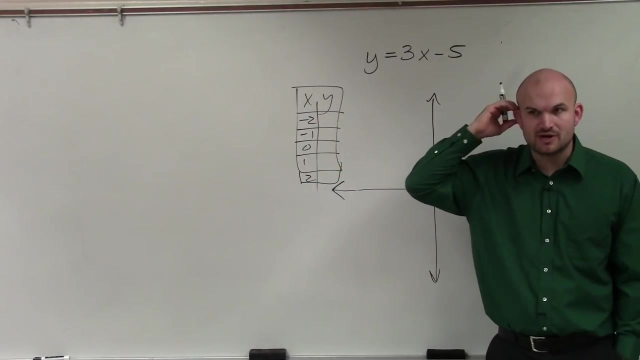 It doesn't matter as much for lines, However, for quadratics, for quadratics and other functions, it actually does matter, And when we get into that I'll explain why it matters. But for right now you can just always use a basic table, But once we get into quadratics, using the table of values, that 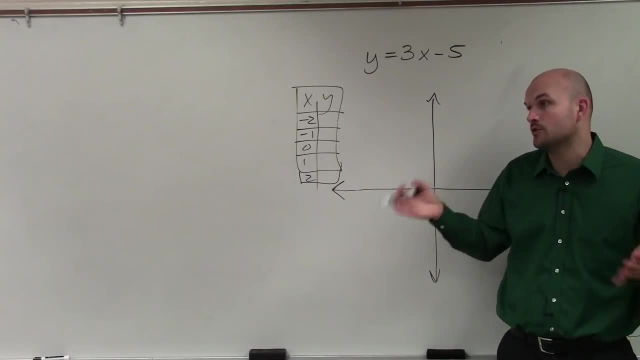 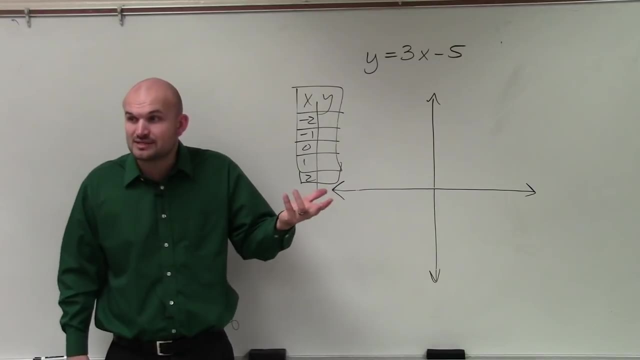 I give you might actually be harmful, might not work, But we'll go over strategies on how to choose the right table when we get to them, But for right now, if we're just looking at a table, we only need two points. 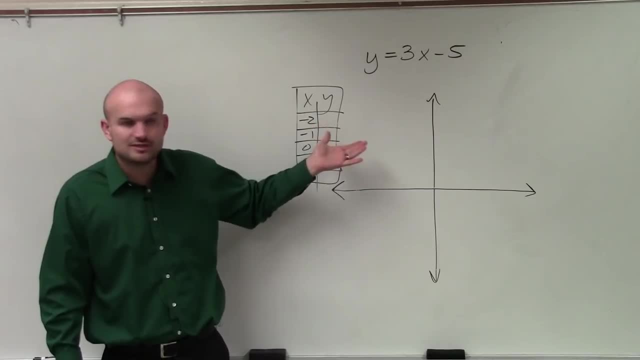 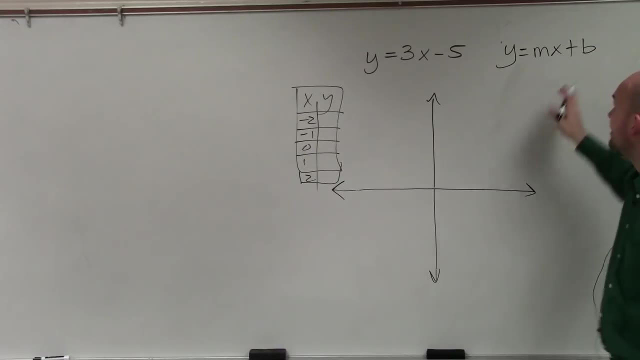 So why go through this whole method of doing this when we only need two points? So I want to go through with you guys how to graph using slope-intercept form, And that is when your equation is set up, when your y variable or your value of y, 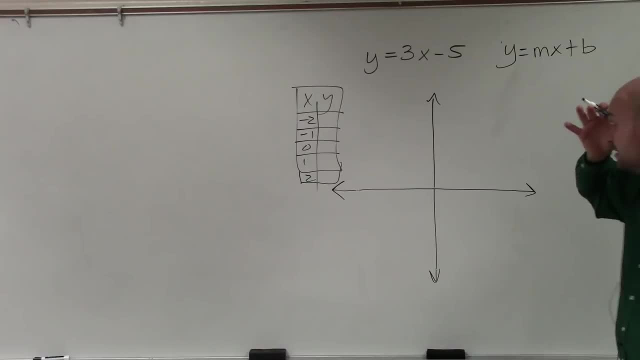 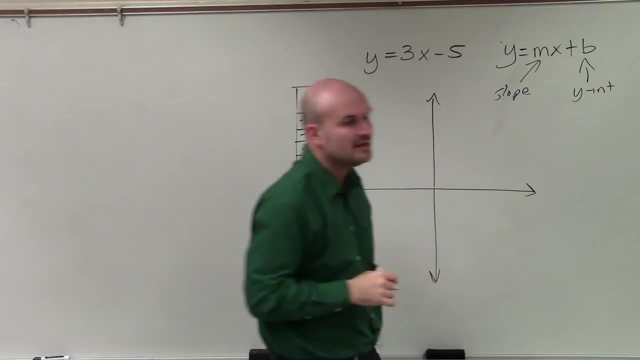 is set equal to mx plus b. So an important thing you guys need to remember is: this is our y-intercept and this is our slope, And I really want to make sure everybody understands, just like domain and range, what is the difference between the y-intercept? 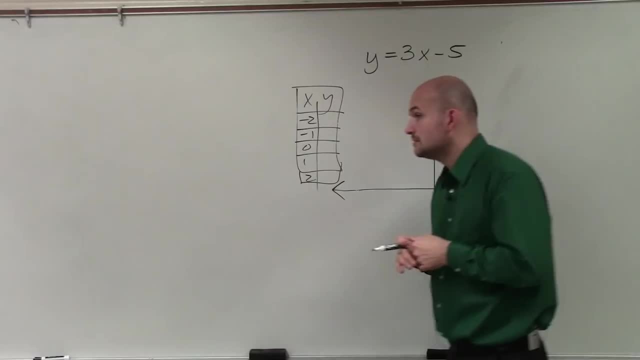 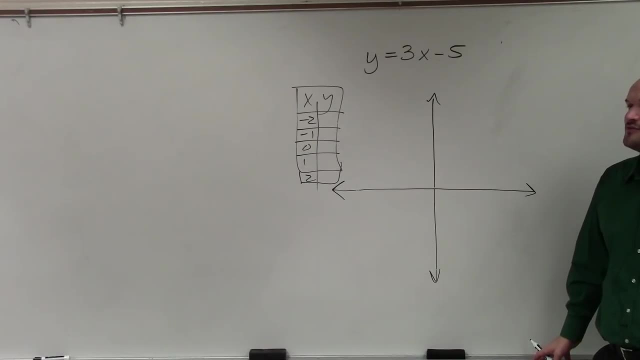 to use all those points. Yes, It doesn't matter as much for lines. However, for quadratics and other functions it actually does matter, And when we get into that I'll explain why it matters. But for right now you can just. 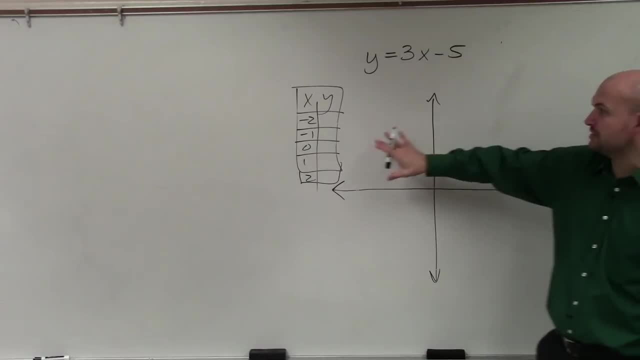 always use a basic table, But once we get into quadratics, using the table of values that I get is just funny, Because then I can actually do shadow métric by adding all my 0's and I can go right over just one thing. 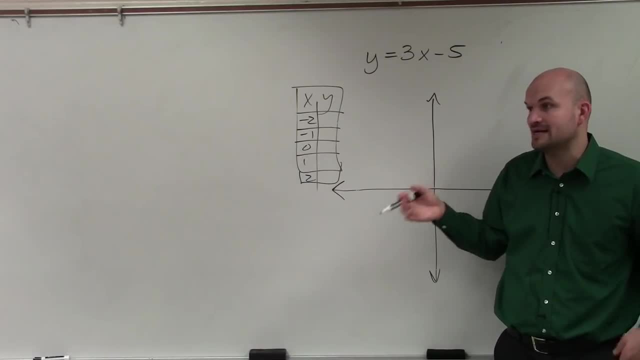 So change, ask shift charge. So how do you get your order of terms and eggs in here I give you? might actually be harmful, might not work, But we'll go over strategies on how to choose the right table when we get to them. 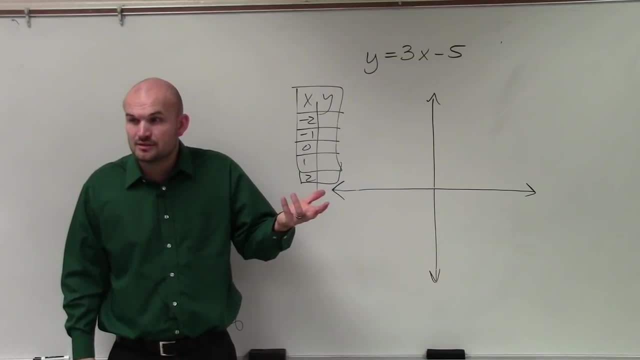 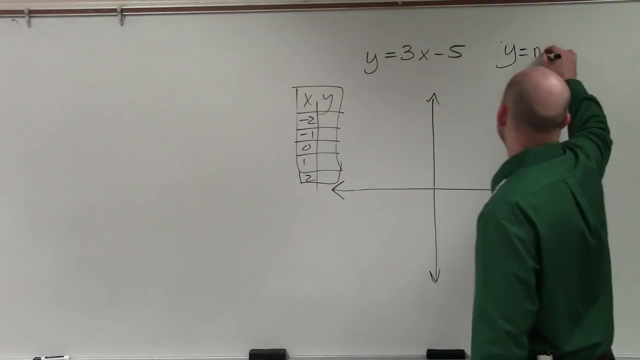 But for right now, if we're just looking at a table, we only need two points. So why go through this whole method of doing this when we only need two points? So I want to go through with you guys how to graph using slope-intercept form. 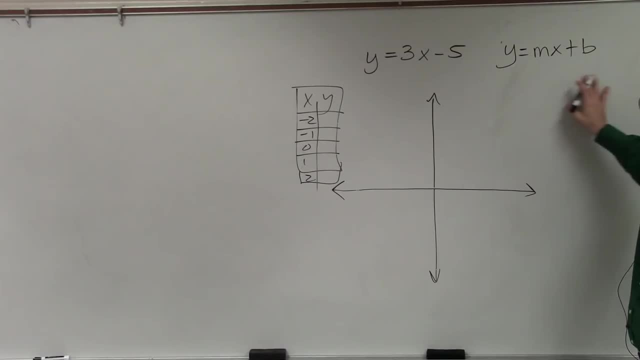 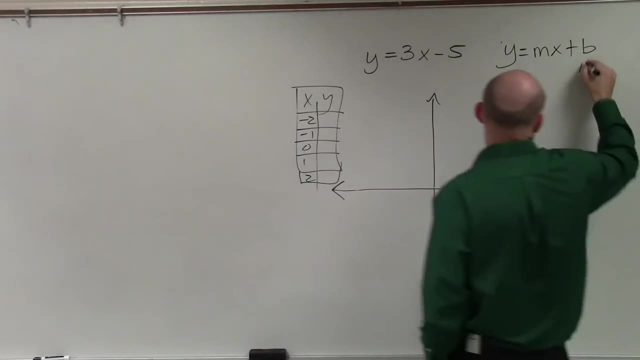 And that is when your equation is set up, when your y variable or your value of y is set equal to mx plus b. So an important thing you guys need to remember is: this is our y-intercept and this is our slope. 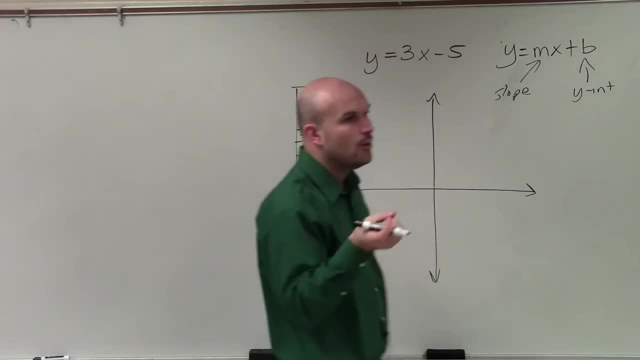 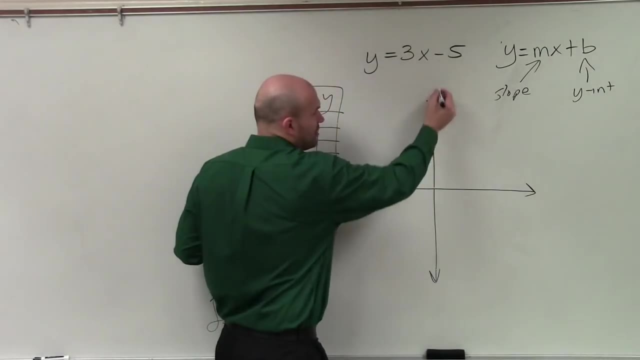 And I really want to make sure everybody understands, just like domain and range, what is the difference between the y-intercept and what is the slope. First of all, the y-intercept is a point. It is a coordinate point on the y-axis. 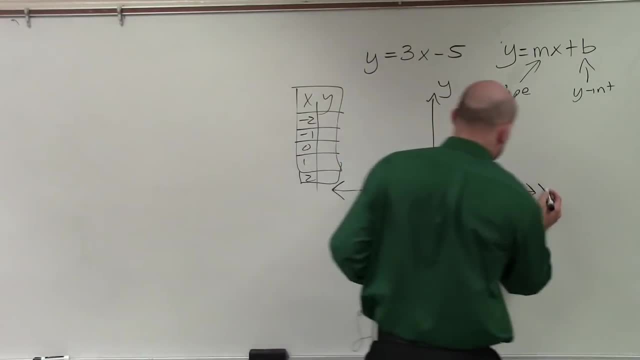 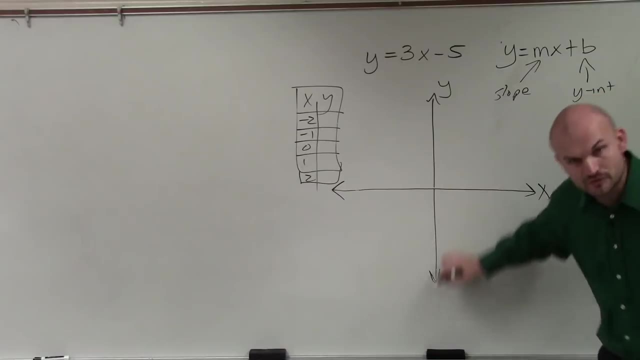 So when I give you the point, do not go on the x-axis, Do not go. Do not go left or right. It is up or down. Here's 0.. If it's positive, you go up. If the y-intercept is negative, you go down. 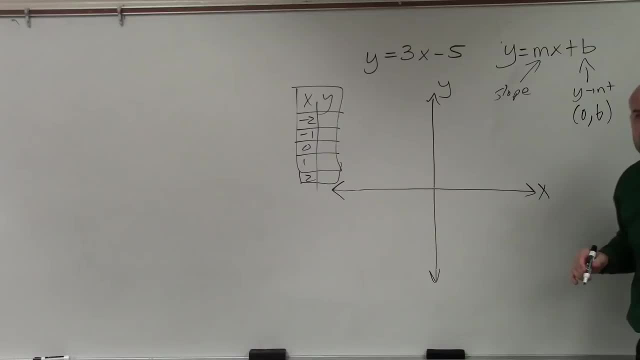 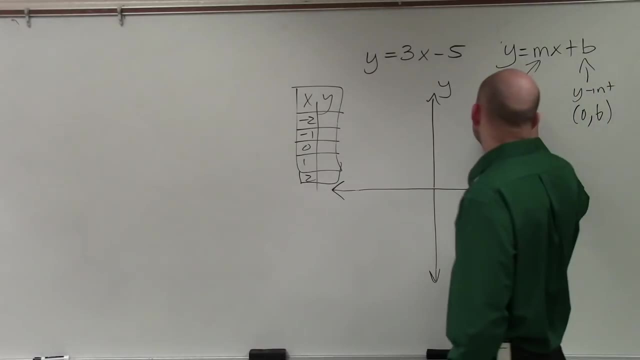 So this is a point. The coordinate point is 0 comma b. The x value is always 0. So you're just going up or down from there. The slope is a ratio. We've talked a lot about ratios, especially for those ACT SAT problems. 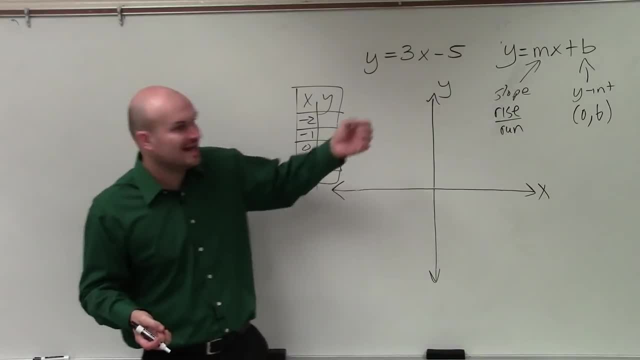 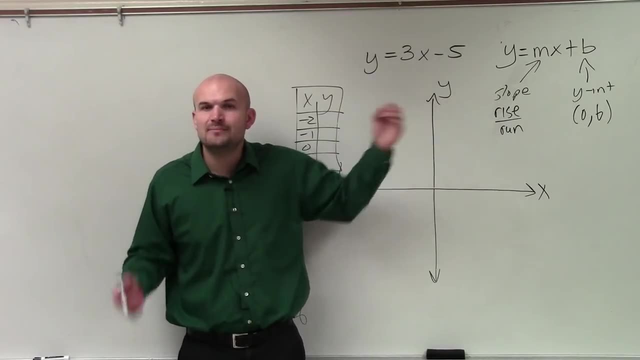 It's a comparison. You are comparing the change in the y values, which sometimes we'll call run. The slope is a ratio between the change in the y values, which is 0 comma negative 5, over the change in the x values. 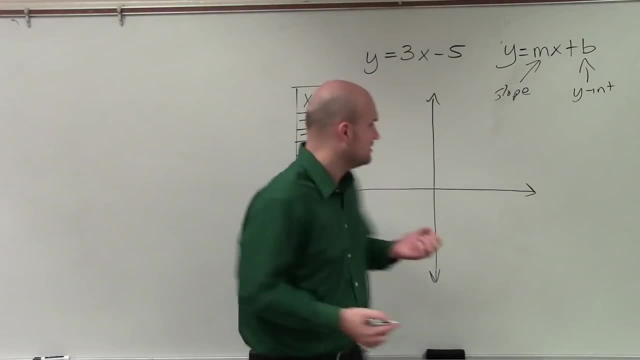 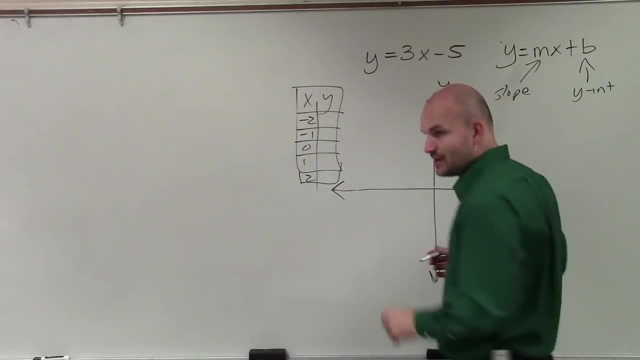 and what is the slope? First of all, the y-intercept is a point. It is a coordinate point on the y-axis. So when I give you the point, do not go on the x-axis, Do not go left or right. 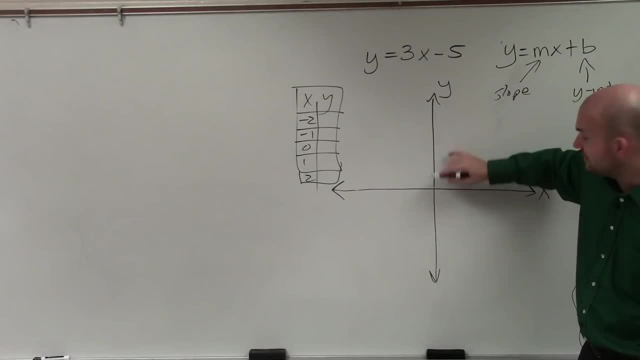 It is up or down. Here's 0.. If it's positive, you go up, If the y-intercept is negative, you go down. So this is a point. The coordinate point is 0, comma b. The x value is always 0.. 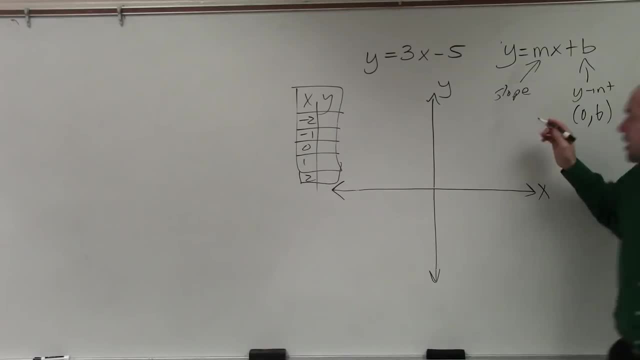 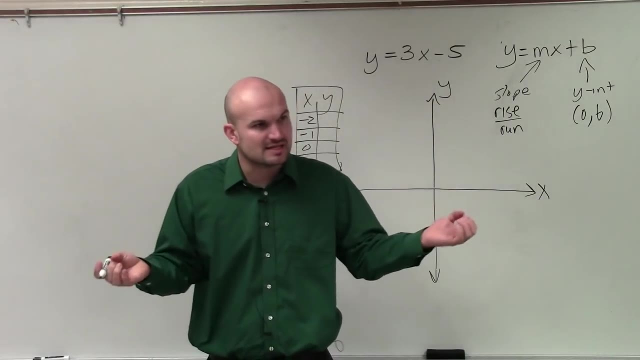 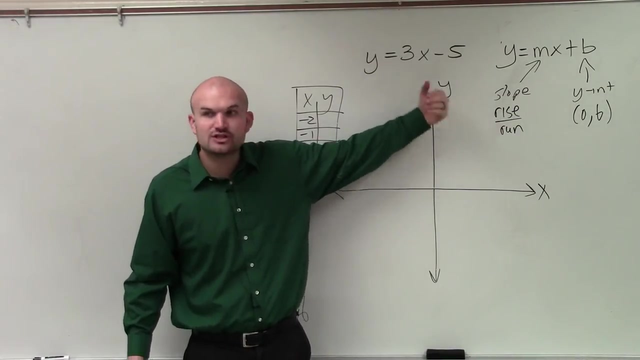 So you're just going up or down from there. The slope is a ratio. We've talked a lot about ratios, especially for those ACT SAT problems. It's a comparison. You are comparing the change in the y values, which sometimes we'll call run, or rise, over the change in the x values, which 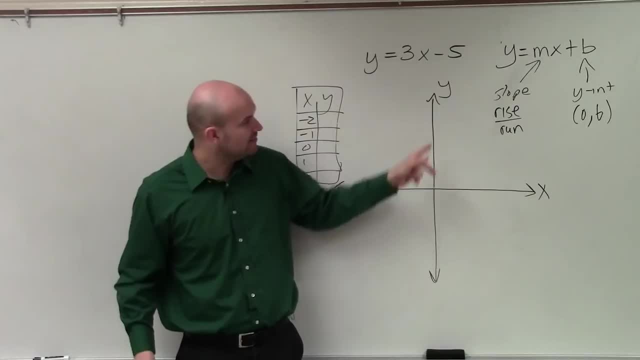 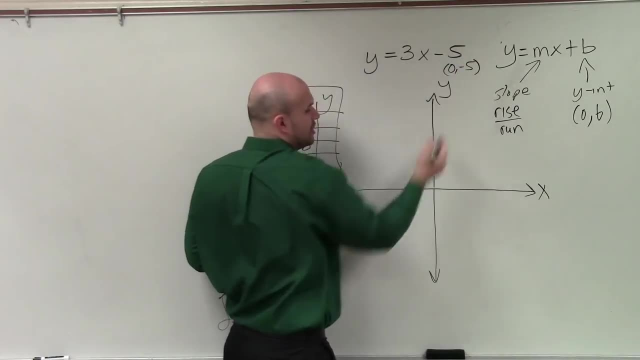 we'll call run between any two points. Now here you can see that I have my y-intercept as negative 5.. So that is 0 comma negative 5.. So I go and plot that: 1,, 2,, 3,, 4,, 5.. 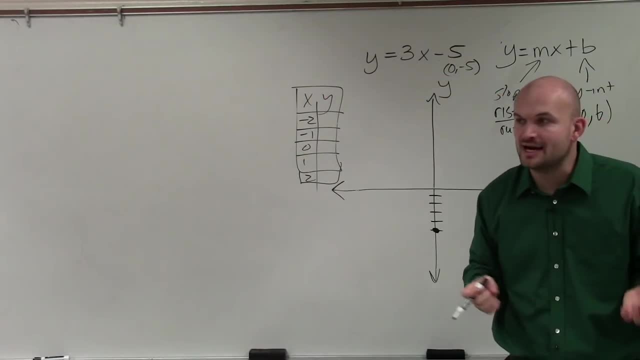 So I've plotted my y-intercept. Now, the slope again, guys, is a ratio between the change between any two points. We only have one point, But we can use the slope to help us find the next point based on that ratio. 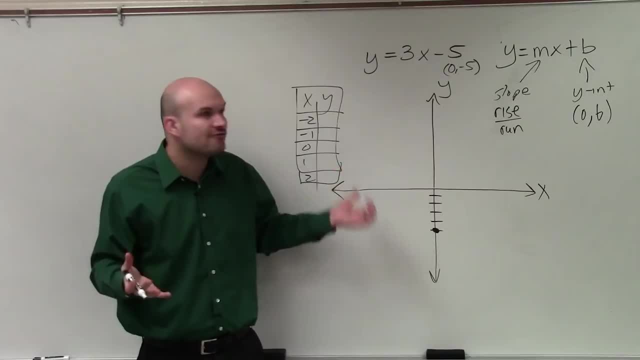 So when you guys are looking at slope, remember it's a ratio, So you want a fraction, This is 3.. This is not in fraction form, So to put it in fractional form, I'll put it over 1.. Now, if I think about this, we're through. 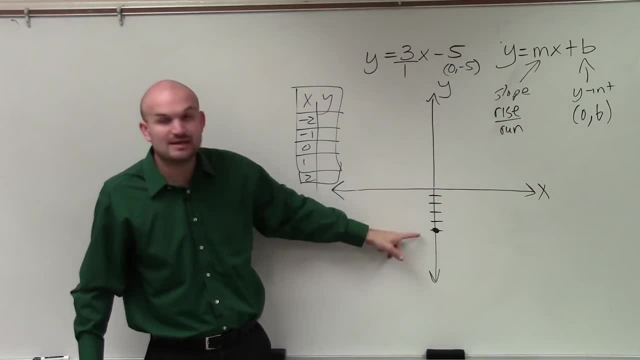 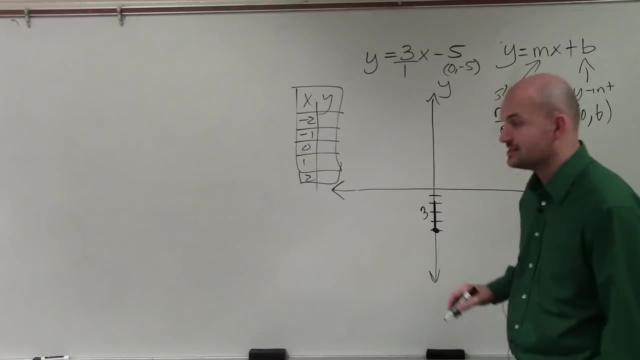 The change in the y values is positive 3. That means between any two points I have a positive change, which is 3.. So I go up 3 units on the y-axis. The change in the x values is positive: 1.. 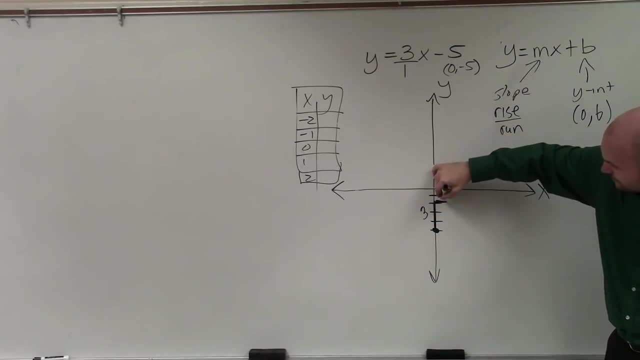 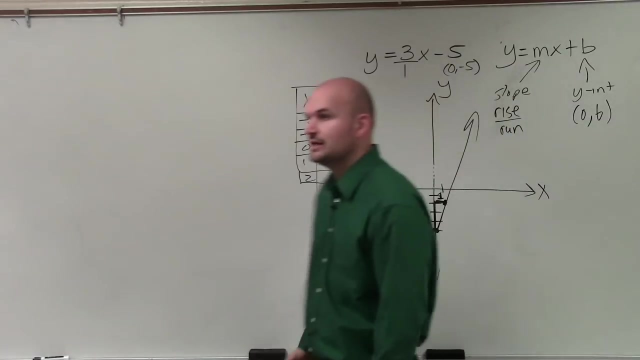 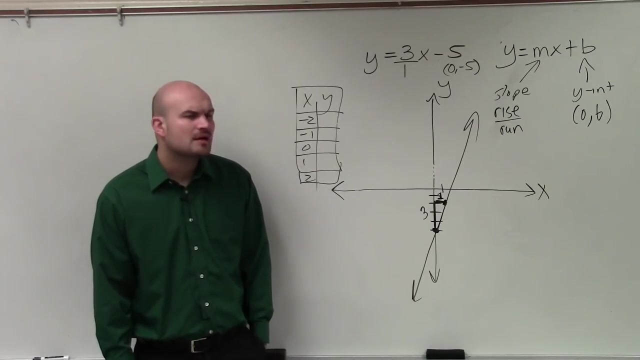 So on the x-axis I'm going to go over 1.. That is going to produce my next point. Now I can connect those two points and create my graph. Anybody have any questions? Yes, I'm sorry, Put it here. 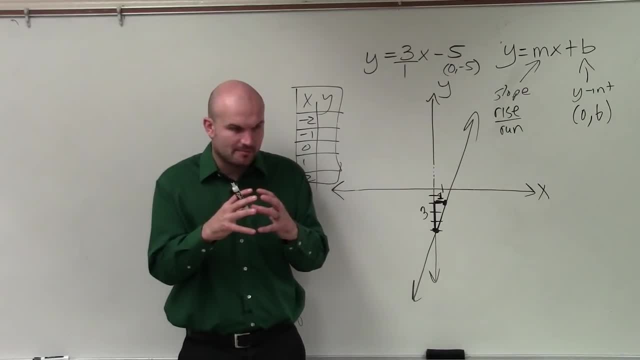 Yes, But what I'm trying to say is: Remember, it's a comparison, It's the change between any two points. So to go from this point to that point, I have to go up 3.. To go from this point to the next point, I have to go up 3..